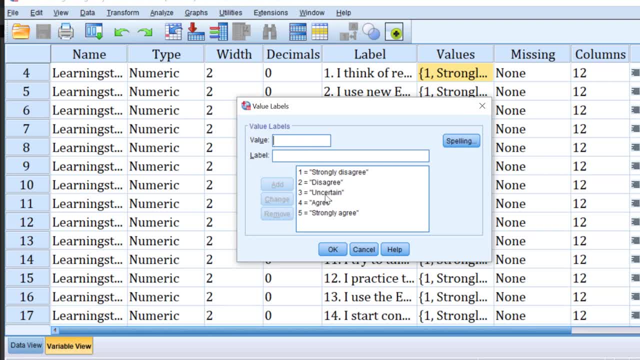 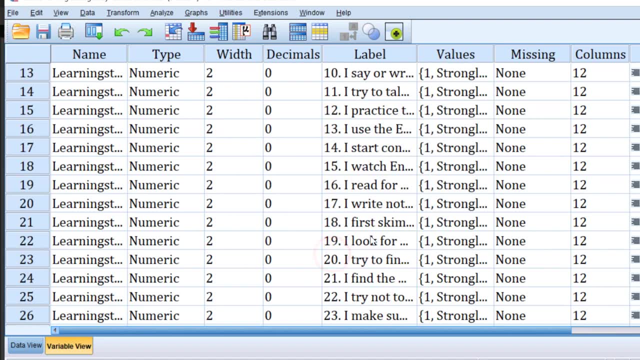 As you can see, one strongly disagree, two disagree, three uncertain, for example, four agree and five strongly agree. So we need to do this for all the items And once we finish, we simply add the code, as you can see, and the label. 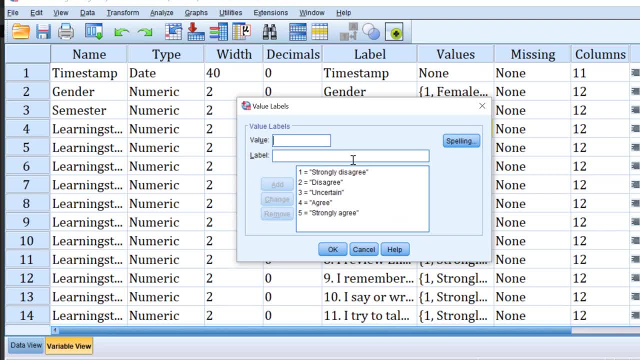 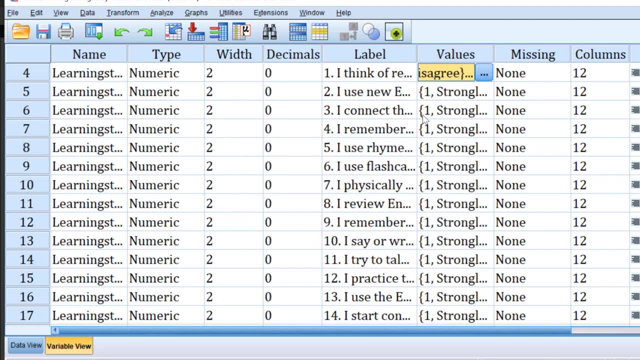 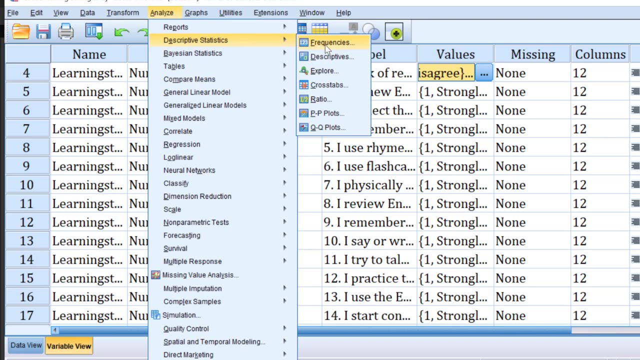 So coding is like a double process, so we do it multiple times. Then once we finish the coding, we can do the descriptive statistics. And to do descriptive statistics we have like this function of add, So we can go to analyze and then descriptive statistics and then we can choose either frequencies or descriptives. 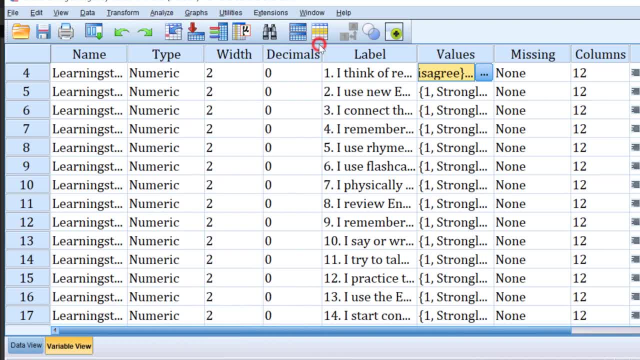 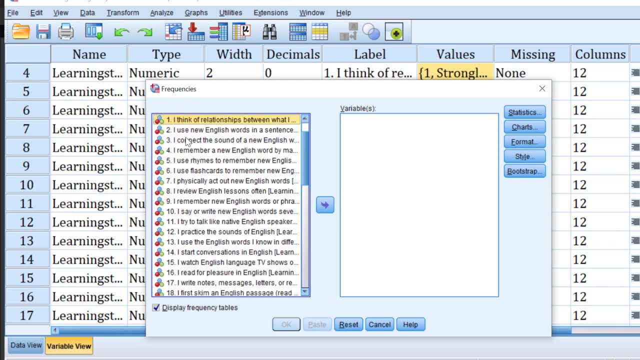 So I prefer to choose frequencies because it's more advanced, So we can go to frequencies and then I can move the items. So here I can move item one, item two, item three, et cetera, till I finish. 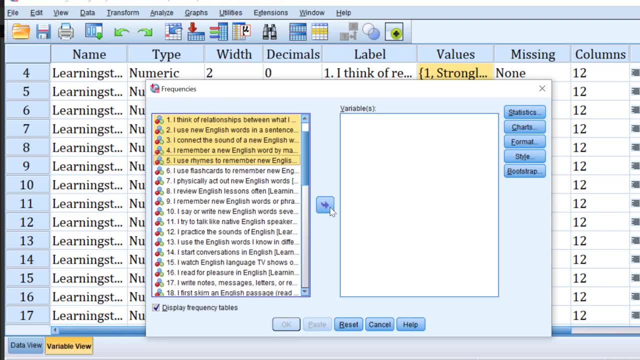 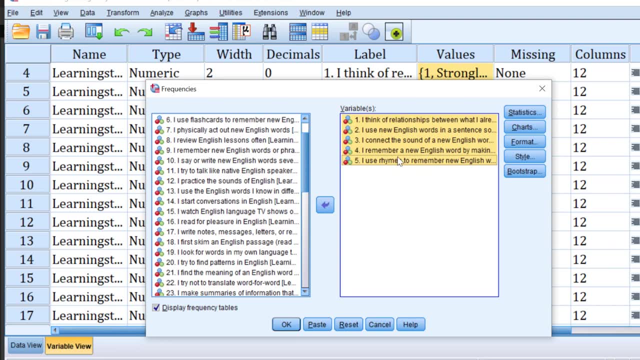 I want just to analyze these five items so I can just move them to the variable view. So I keep just clicking on it, I click in control and then select each item separately. Then I go to statistics and then I can choose. 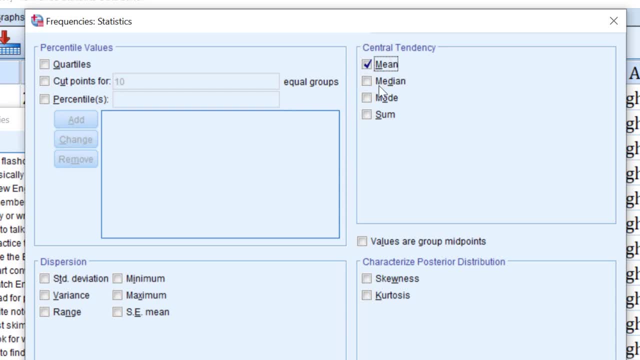 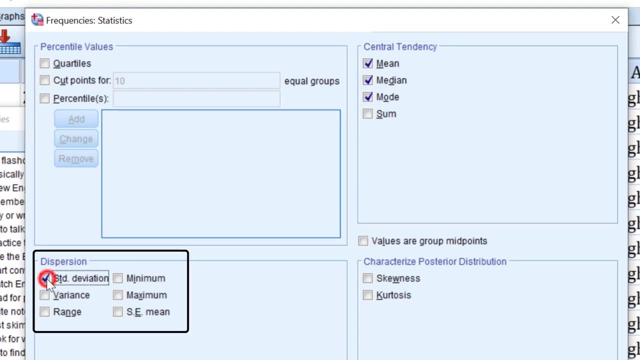 Suppose that I want the mean, like the average, and I want for instance the mode and sometimes the median. These are for descriptive statistics and most specifically central tendency measures And for dispersion measures. in descriptive statistics we have standard deviation. 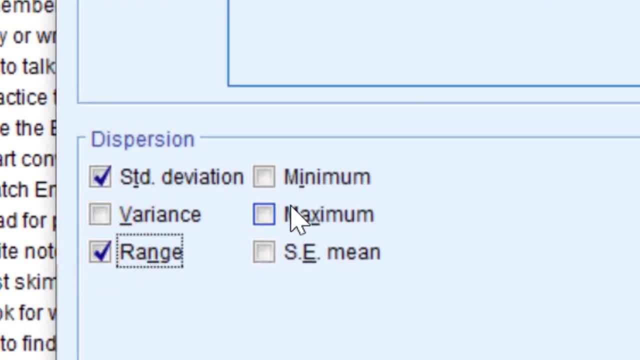 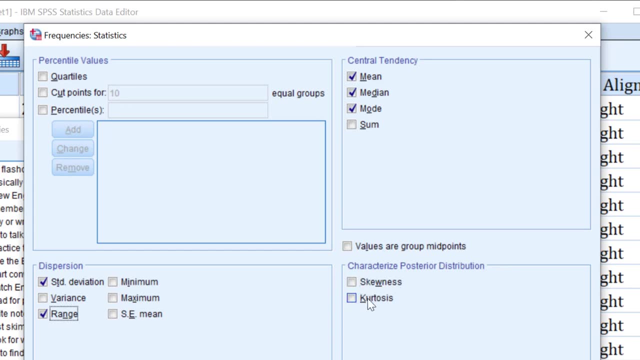 We can choose the range, Sometimes we can choose the minimum, maximum, Et cetera, And we have also kurtosis and skonis with regard to the normality of the data. So, to tell you the truth, mostly Lackert scale. data is not normally distributed, so you can expect to use non-parametric tests as inferential statistics. 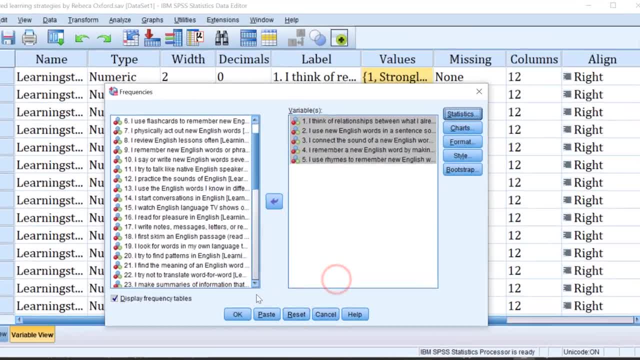 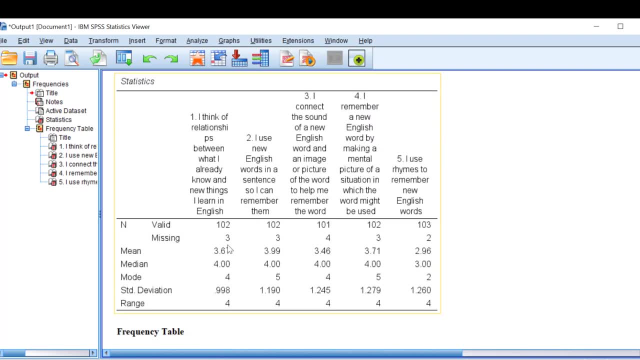 So once we finish, I can click continue and then click OK and wait for the output. So this is the table that contains the Lackert scale items and we have the mean median mode standard deviation range. Now how can we go about the interpretation of this result? 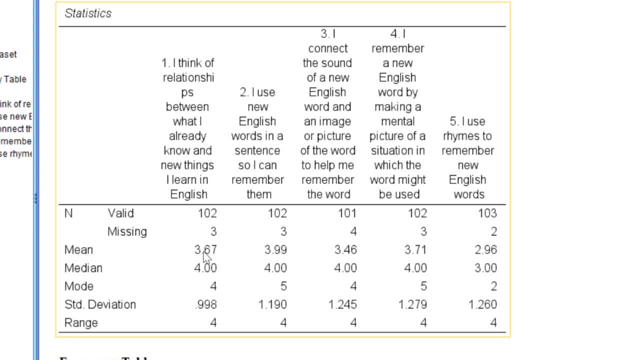 So, as you can see, the mean here ranges from 3.67 to 2.96.. So what do those values mean? You remember the coding? So we coded: 1 as strongly disagree and 5 as strongly agree. This means that the higher the mean score, the more agreement is expressed with each statement. for instance: 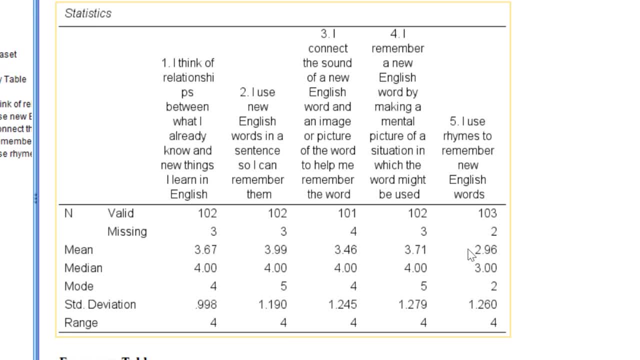 But we can rank these statements. for instance, We can say that the first statement is that it has received a higher rate of agreement, mostly uncertainty. So we have this statement of 2.. I use no English words in a sentence so I can't remember them. 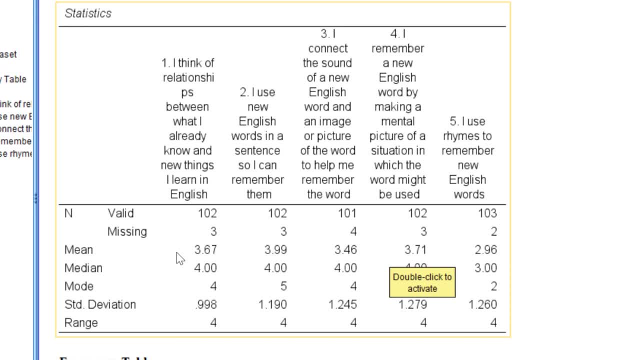 So most respondents do this, et cetera. So I can just rank these items based on the mean score, And the higher the mean score, the more agreement that is expressed with each Lackert scale item. Then we have the median, That is the midpoint value. 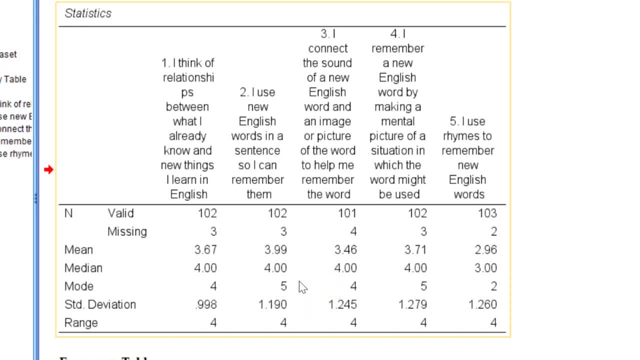 We have the mode That is the most frequent value. So here, 5.. This means that most respondents strongly agree. And then we have 5- again Most respondents strongly agree. as you can see, The standard deviation just tells us how the respondents differ in terms of their attitudes with regard to certain issues. 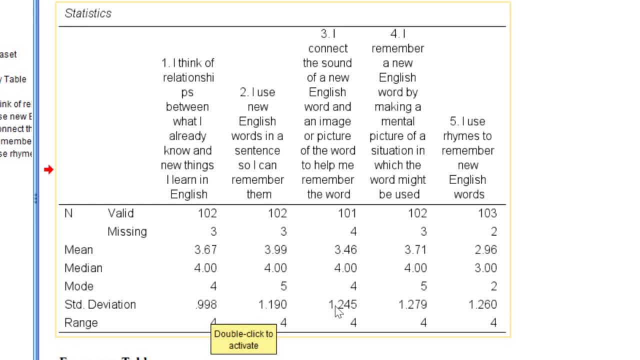 So the higher again the standard deviation, the more heterogeneous the sample is, And the lower the standard deviation, the more homogeneous the sample is. So it's not a matter of attitude or agreement or disagreement et cetera. So we use just both, the mean especially and the standard deviation. 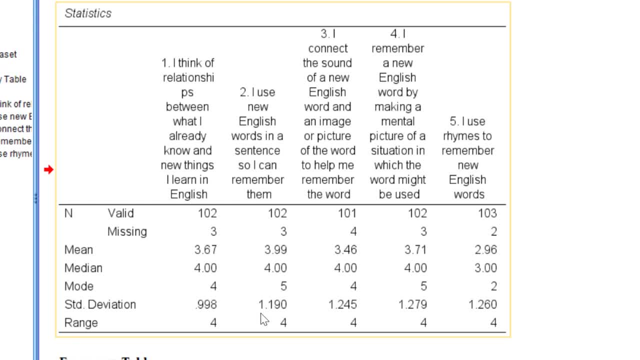 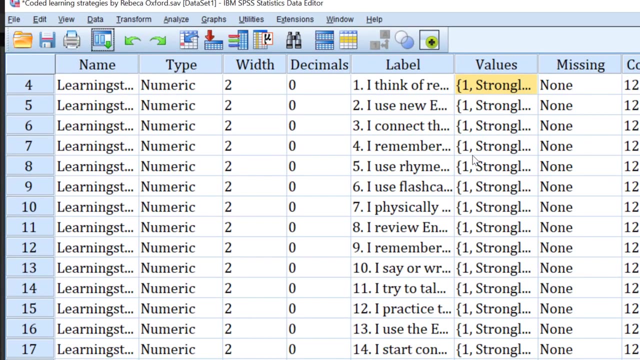 The mean for central tendency measure and standard deviation for dispersion measure when it comes to descriptive statistics. So once we finish descriptive statistics, we can go for inferential statistics. So why do we use inferential statistics? We simply use inferential statistics to generalize the results from the sample that we have to the whole sample. 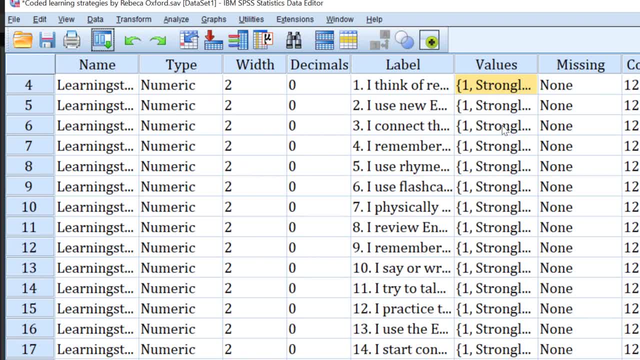 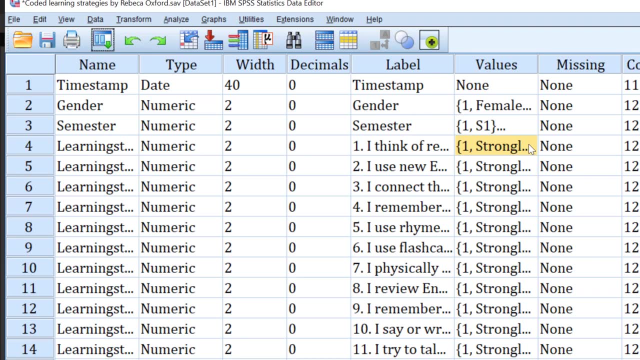 That we have to the whole population, Given the p-value that is below 0.05 or 0.01 or 0.001.. So it depends on the threshold level that is determined. So we have different inferential statistics. We have the parametric and non-parametric tests. 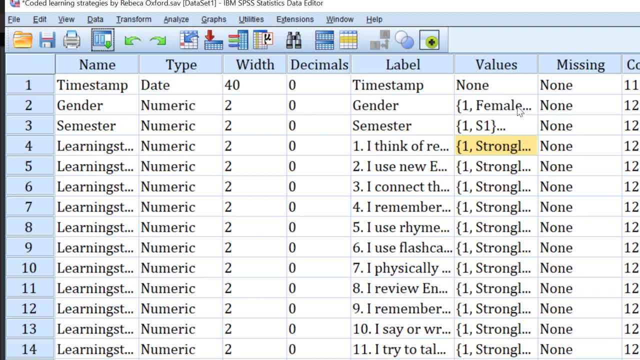 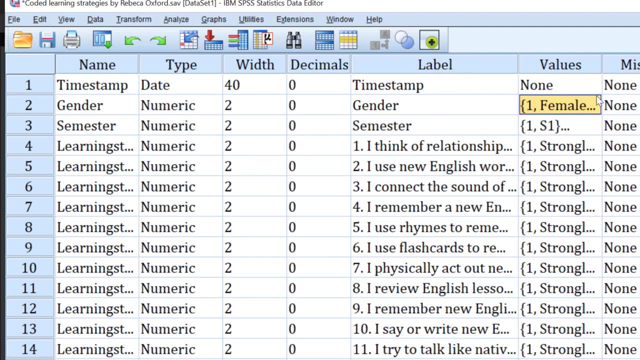 For the parametric tests, we can go for the independent sample t-test, Let's say to compare gender- male and female- respondents, along with the strategies that you use, Like who use this strategy, for example, more male or female, et cetera. 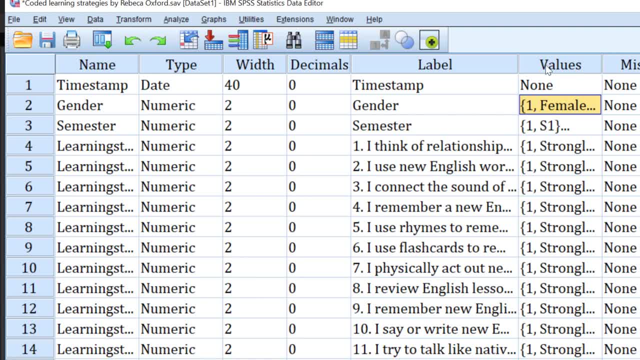 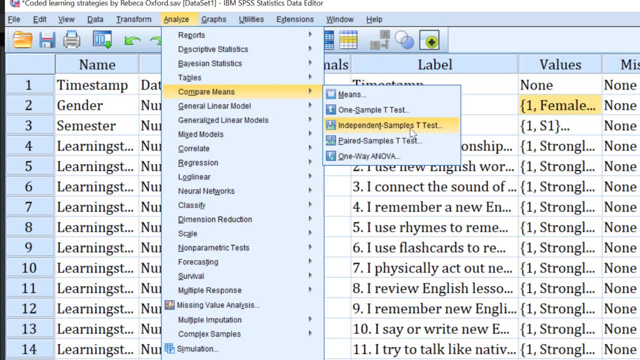 So this is called the independent sample t-test. Again, to do this we can just go to analyze and then we go to compare means and we go to independent samples t-test And then we put gender as the grouping variable and we assign. 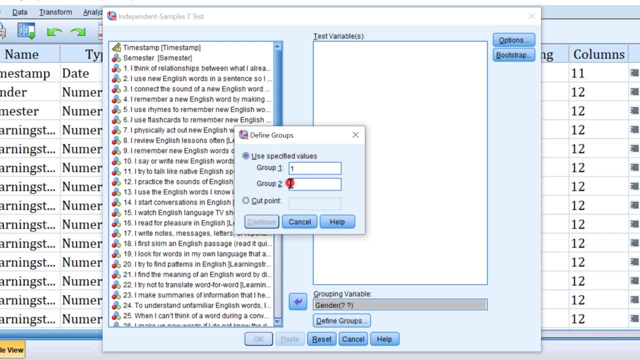 So again, the coding is always important. So one for group one And two for group two And click continue. And I put, for example, this statement, Like I remember new word or new English word, by making links, for instance: 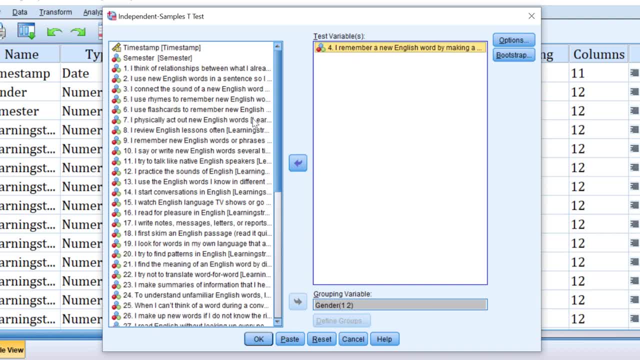 And then I click OK. I just want to see this statement: You can choose all the items together. Sometimes you can combine items together. That's yet another strategy that you can use. So it mainly depends on your research questions, your research objectives and your research hypothesis. 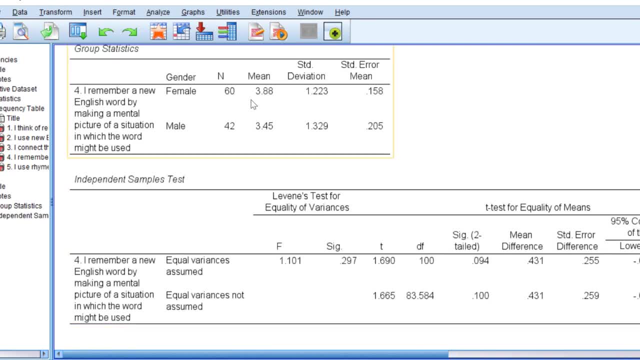 So again we click OK And wait for the output. Here it is. So again we have the descriptive stats within the inferential stats. at the same time We have female, We have the N that refers to the sample size, So we have 60 female respondents and 42 male respondents. 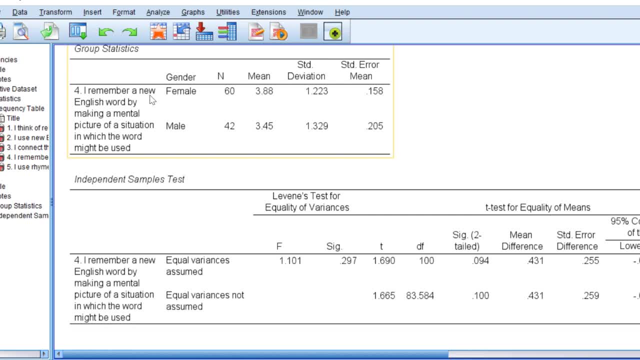 The mean score here differs from male to female with regard to remembering an English word by making a mental image. So here the mean score of female respondents is higher than that of male respondents. Therefore, female respondents agree with this statement more than male respondents do. 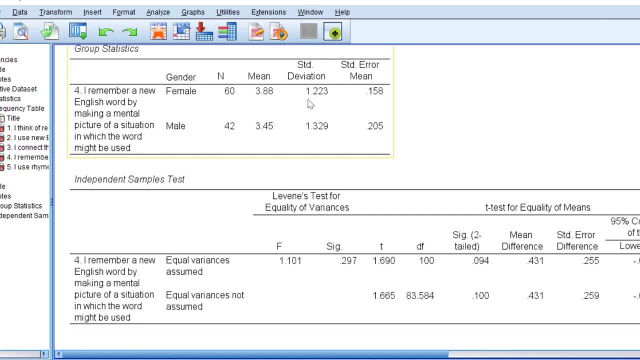 And standard deviation. you can see just the difference in terms of, or the divergence in terms of, expressing the attitudes. And then let's look at whether this difference is by chance or is statistically significant. This means that we can generalize this finding from the sample to the whole population. 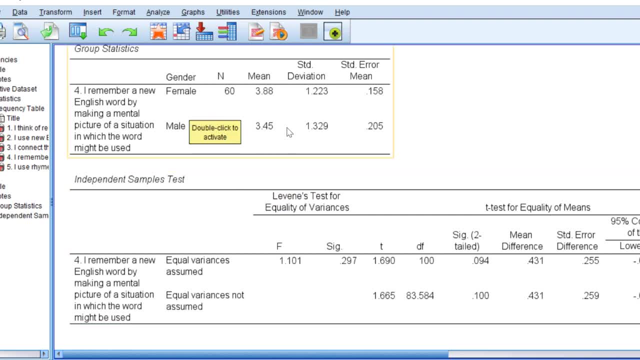 Is this really scientifically true? Is there really Is scientifically a difference between male and female with regard to making mental picture? I don't think so. Maybe if you are a psychologist, you may have more arguments with regard to this. So anyways, so we have sick two-tailed. 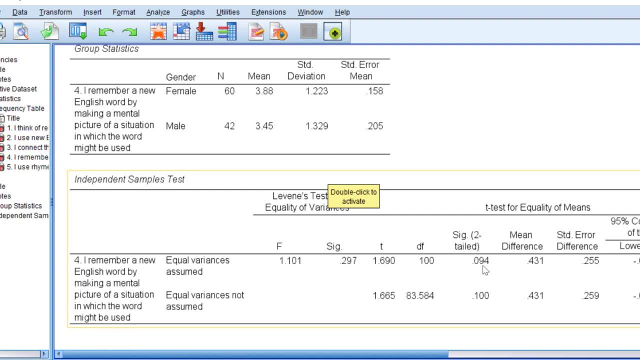 This refers to the p-value. You remember, if the p-value is below 0.05, this means that there is a statistically significant difference. If it's above 0.05, this means that there is no statistically significant difference. And usually we have two sick two-tailed. 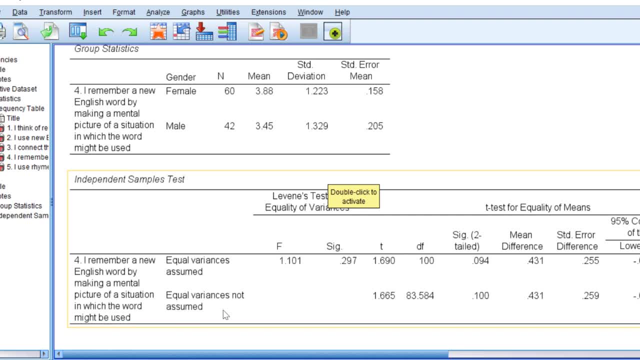 We have male. Equal variance is assumed and equal variance is not assumed, So we can go for both of them. As you can see, the p-values for both are not statistically significant since they are below point. So they are not below, They are above 0.05.. 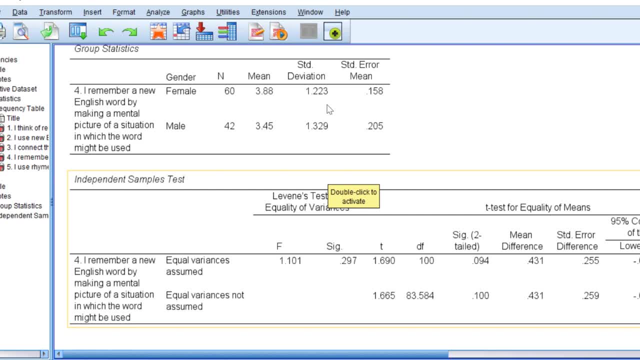 This means that we cannot be sure 95% that this difference that exists between male and female respondents with regard to remembering a new word by making mental picture is statistically significant And therefore we reject the null hypothesis, Not reject, rather, We fail to reject the null hypothesis that assumes that there is a statistically significant difference between male and female respondents. 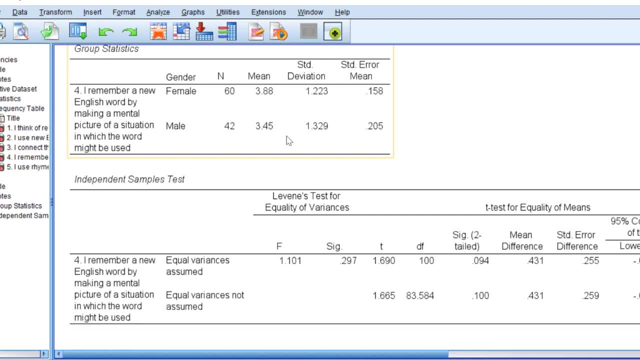 Okay, Because we have the null hypothesis. that assumes that there is no statistically significant difference. So we either reject it in favor of the alternative hypothesis or we fail to reject it, Okay. So we don't say support or not support. We say just reject or fail to reject. 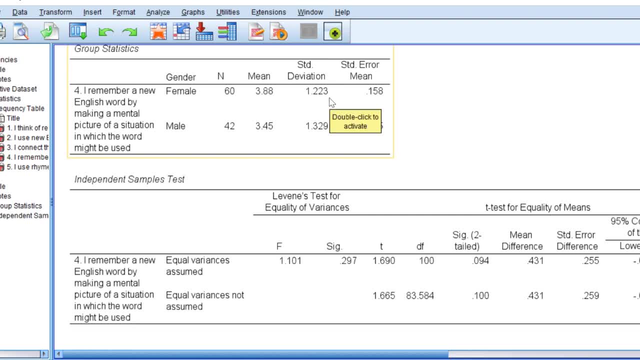 Okay, So we do this without testing the normality, because I know that the normality is not that accurate, because we are dealing with social science and attitudes are divergent from one person to another. But to avoid this issue- whether to use parametric or non-parametric tests- I can just use sensitivity analysis by using both parametric and non-parametric tests, like the independent sample t-test and the Mann-Whitney U-test. 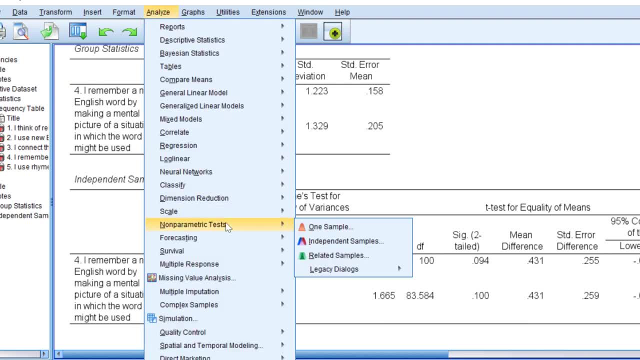 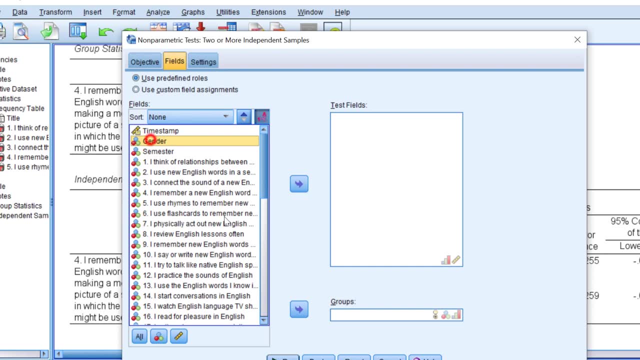 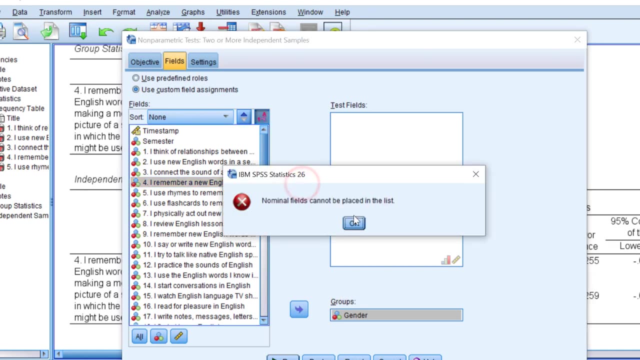 So to use the Mann-Whitney again, you go to analyze and you go to non-parametric test. Okay, So you go to non-parametric test and you go to independent samples- t-test or Mann-Whitney U-test- and we go to gender and move it to groups and this statement and we put it here: 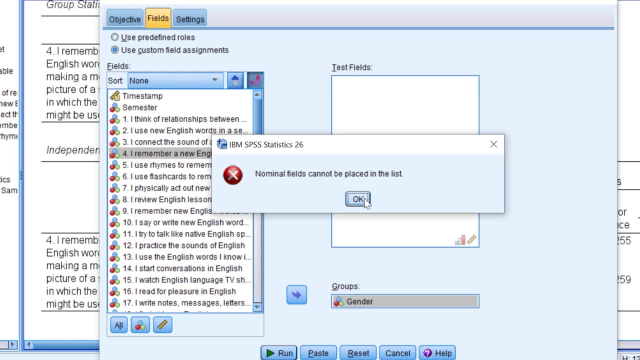 But nominal fields cannot be placed in the list. So what we need to do here is just change the measurement level, because, as you know, we have ordinal interval, ratio and nominal scales, Or rather measurement levels. Okay, So we need to change the measurement level. 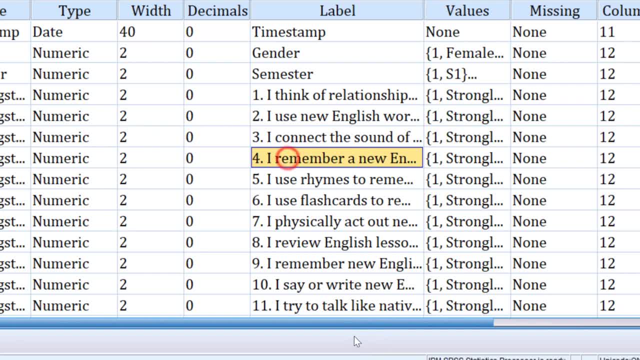 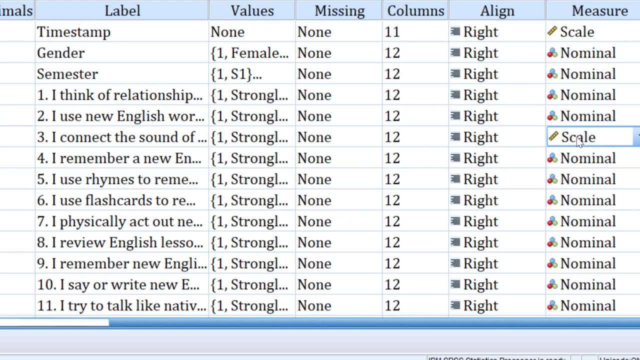 To do this. we can just go back to a spaces, look for four and go for the measurement level From nominal. we can change it to scale, because some students or researchers ask me why we have those. let's say measures are nominal or scale or ordinal. 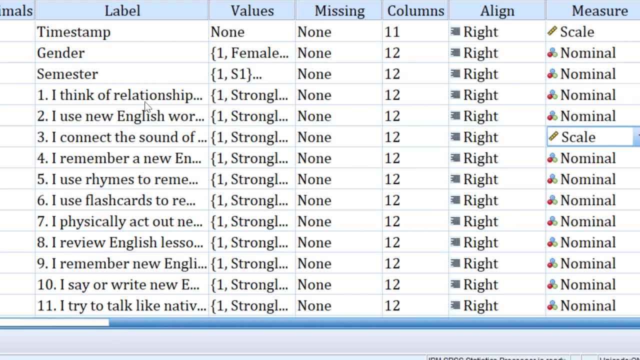 So just forget about what you are reading about lacquer scale as being ordinal. that depends truly on your research objectives and your research questions and what you actually want to do with it. you can consider it nominal, ordinal interval, whatever you want, depending on the analysis. 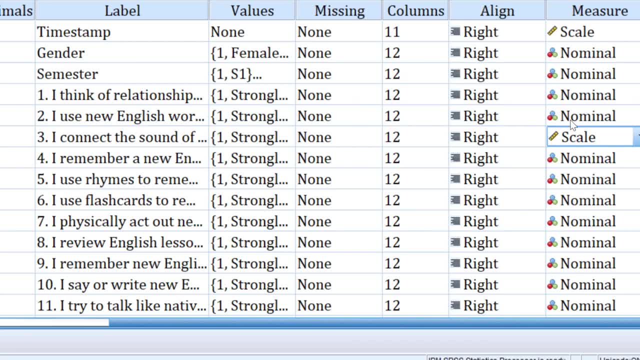 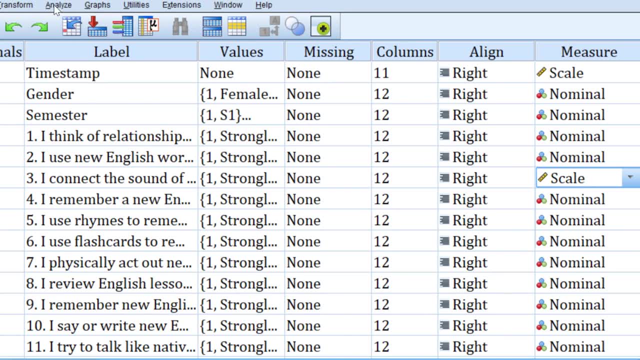 that you want to run. so once we change it, because a species is another story, so a species has different criteria, so to speak. okay, so anyways, we can just go to uh, analyze, uh, then non-parametric tests, independent samples, t-test, and so just go back to this, so we have independent samples. 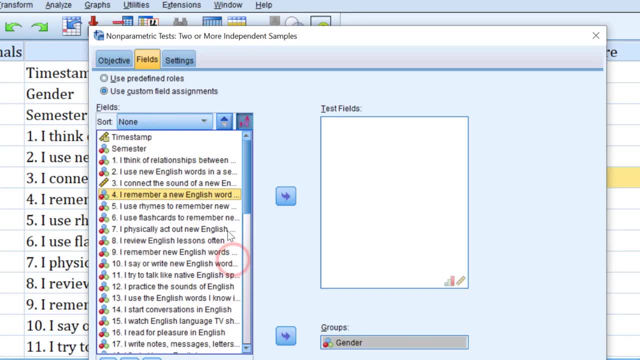 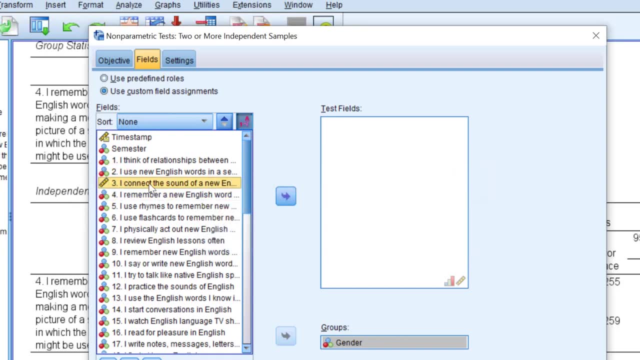 t-test. we have non-parametric independent, so i move this okay, for example. so i change to. so, for the sake of illustration, i can just move, uh, this statement number three, rather not two, to this box, just for the sake of illustration. so you know now the how you can do it and i click run again i can. 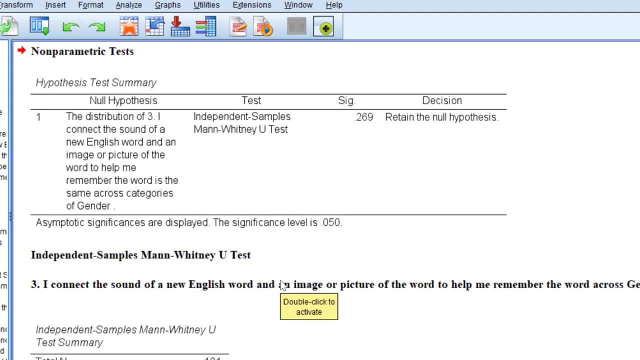 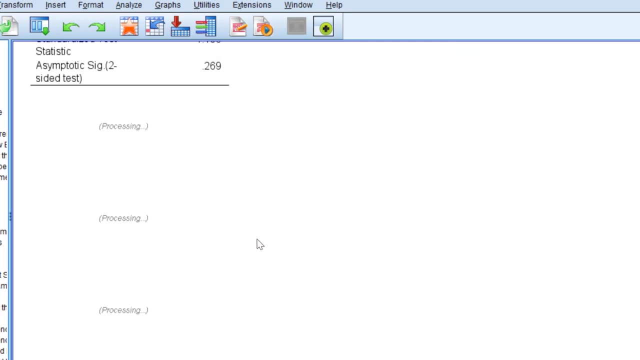 wait for the output. so this is the uh non-parametric test. you see, the value is below, or rather is above, 0.05. it's 26. so we the decision is to retain the null hypothesis and although there is difference- maybe not noticeable difference- between male and female. 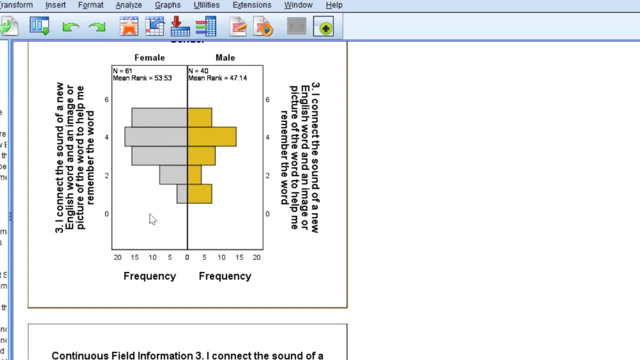 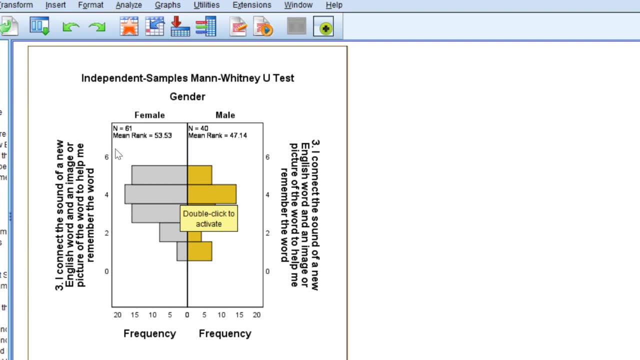 in favor of female respondents. still, this difference is not statistically significant, so we cannot generalize it to the whole population. so this is just one uh, inferential statistic test you can run, for instance, the chi-square test- there are videos on how to do that. the novat test- there are videos on how to do that. uh, the regression tests, and uh, there are some. 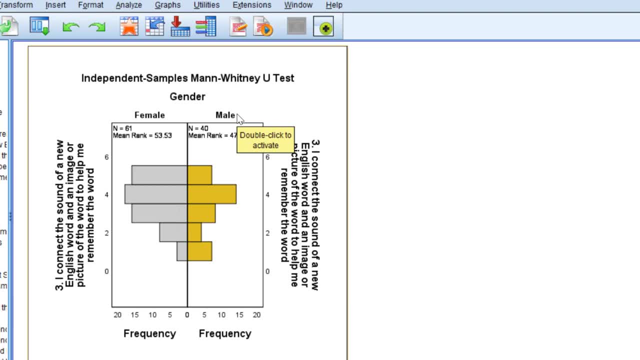 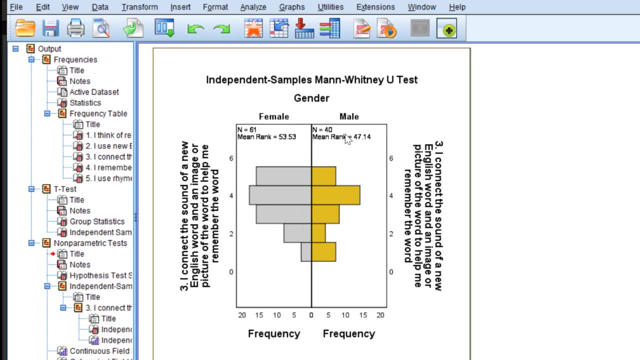 videos on how to do that. i can attach the links to each video separately in the description box. if you have questions or remarks, not hesitate to post them below or contact me via one of my social media platforms. till then, see you in another tutorial. bye for now.